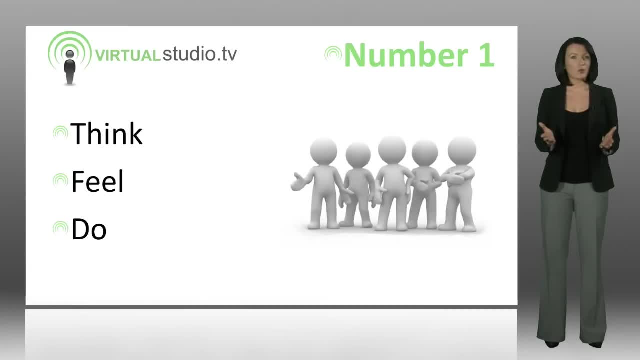 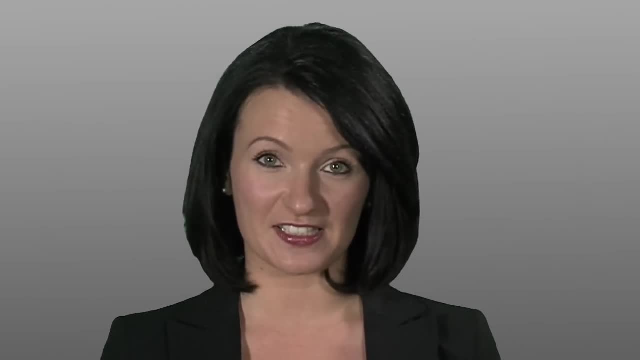 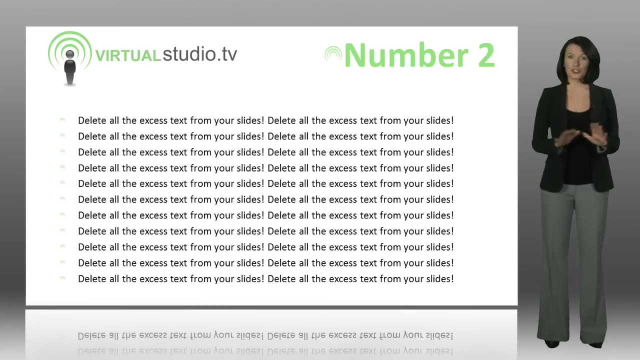 Once you have these clear objectives in your mind, you are on your way to delivering a winning presentation. Number two: delete all excess text from your slides. Loads of bullet points on your slides are a complete waste of time. Nobody actually reads them. The brain is a self-altering mechanism and that's why their focus is so much on the audience, Because the audience is watching, the audience is listening and the audience is listening. So what benefit will the audience get from listening to you? What do you want them to think, feel and do as a result of listening to you? 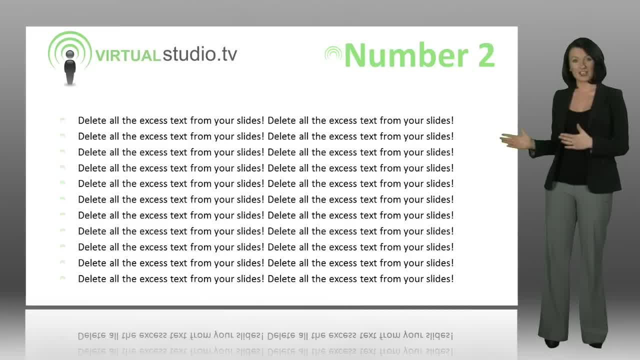 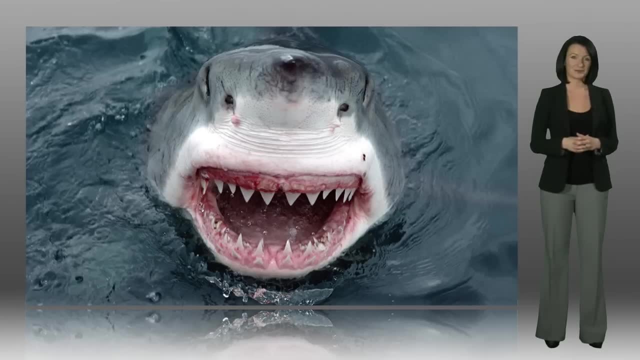 self-organizing mechanism. If you use slides like these, you're sending a signal directly to the audience to start daydreaming. Your slides are not your speaker notes. Use powerful images and pictures. They are much more effective in getting your message across. 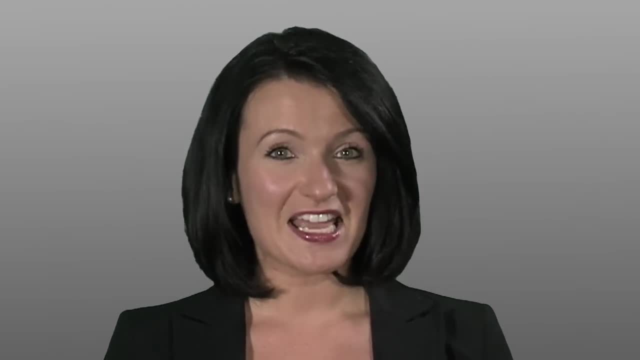 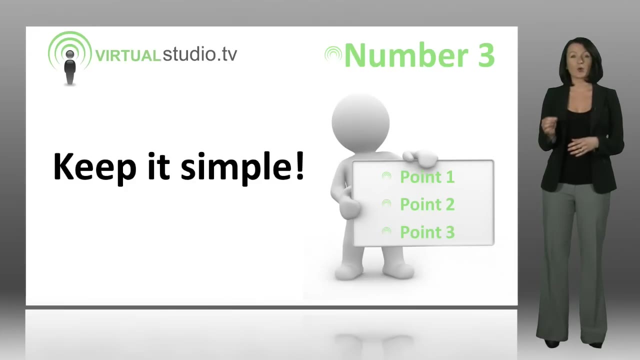 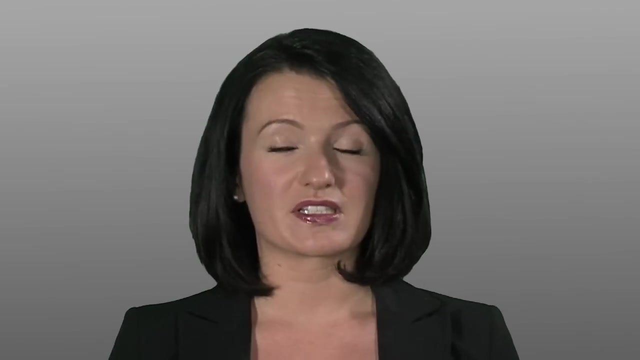 Number three: keep it simple. Less really is more. Get used to cutting out material. Decide in your presentation only what really matters. This is a difficult process, but think back to point one. What do you want the audience to think, feel and do If your 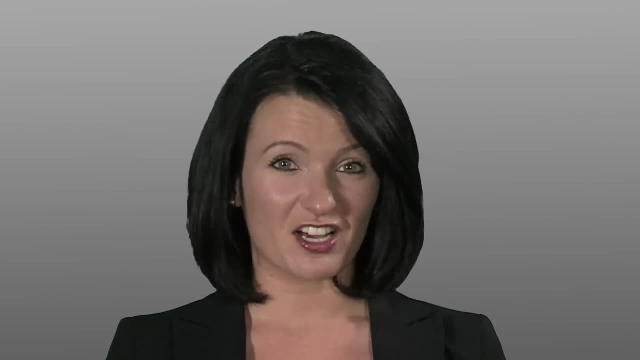 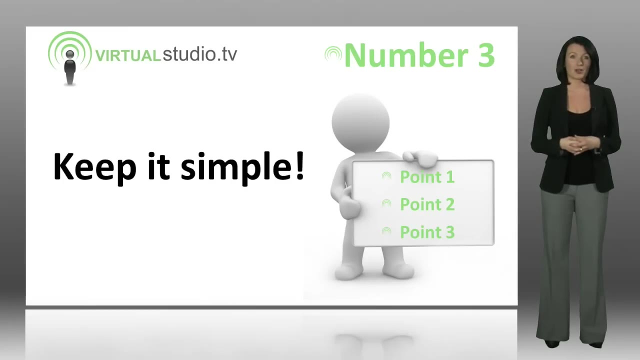 content doesn't match your answers to these questions, cut it out. Use the same language that you'd use while explaining your presentation to a friend in the local pub over a pint, and try to use simple wording, too, to make your content clear and easy to understand. Rule number four: use simple words that are easy to understand and easy to understand. Rule number five: use simple words that are easy to understand and easy to understand. Rule number six: use simple words that are easy to understand and easy to understand. 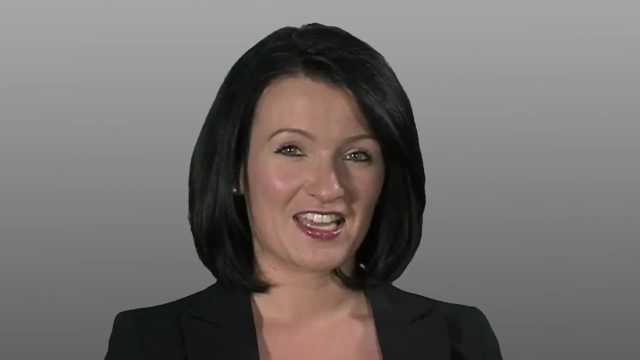 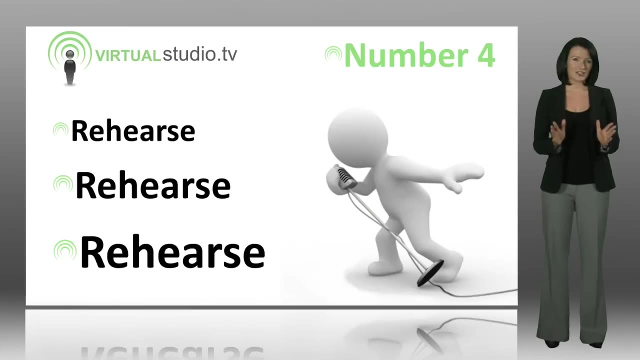 Rules of three can be really effective. Number four: rehearse, Always, always rehearse. The biggest single difference a presenter can make to their performance is to stand up in front of the bathroom mirror and rehearse. If you are serious about success, then you need to get serious about rehearsing. And 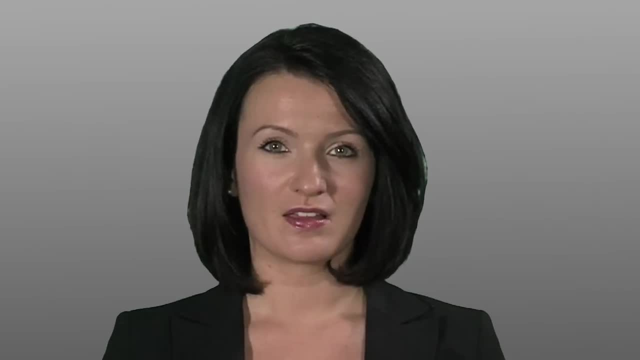 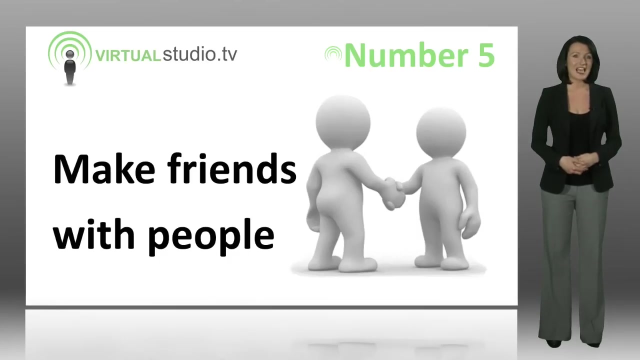 if you don't prepare, then prepare to fail. Number five is especially important If you are speaking at an event or away from your usual place of work. make friends with the crew and the people at the venue. The crew can play a huge part in your success And 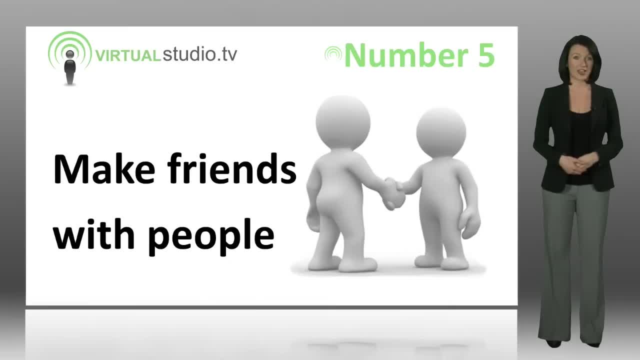 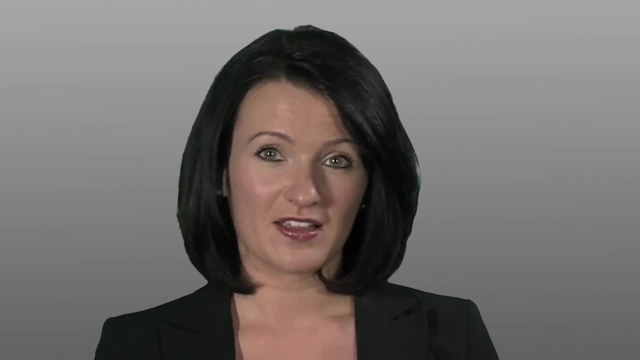 if you are rude and arrogant, they'll enjoy watching you fail. Get there early, make friends with them, learn their names and ask them for help and advice. Ask politely for a sound check. Ask to view your PowerPoint slides on the big screen. You can see where I'm going. 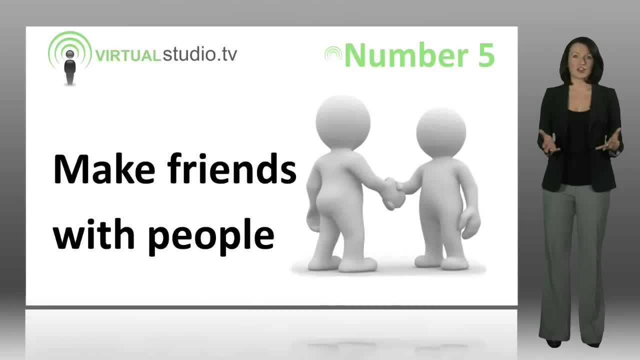 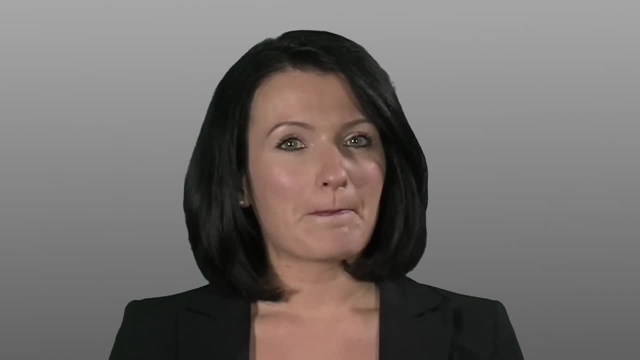 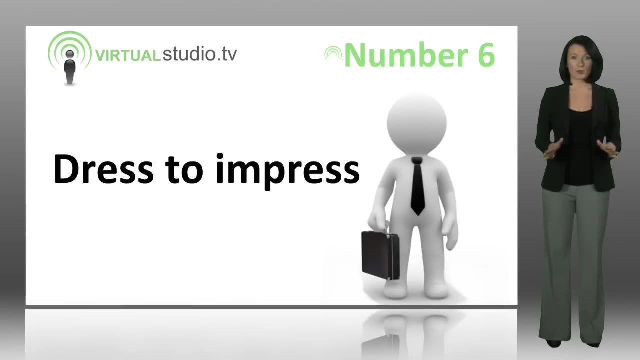 with this. This preparation will ease your nerves and raise your confidence before your presentation starts. Number six now. this is a much debated point, but we always say: dress to impress. If you are in any doubt about what to wear: be smart, Smart hair, smart shoes, smart dress sense. 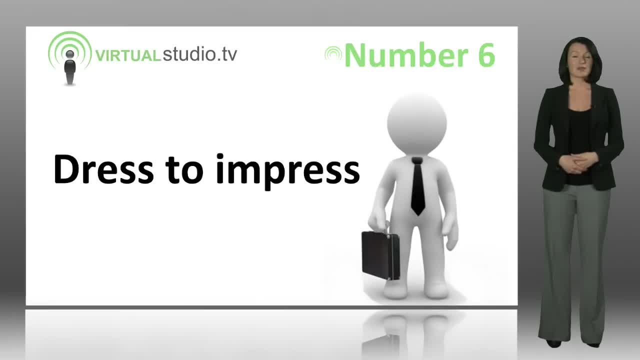 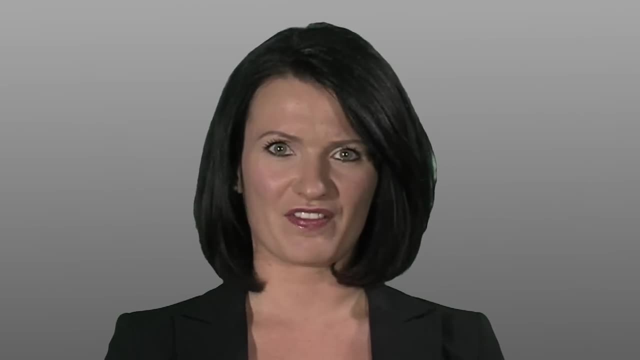 Don't fall into the trap of getting up on stage looking casual, because you'll only look scruffy If it's smart casual dress wear. always go the smarter side of casual. Better for people to say, wow, she looks smart rather than God, she could have made an effort. 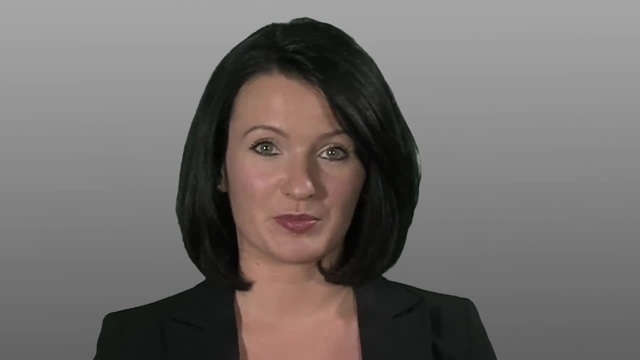 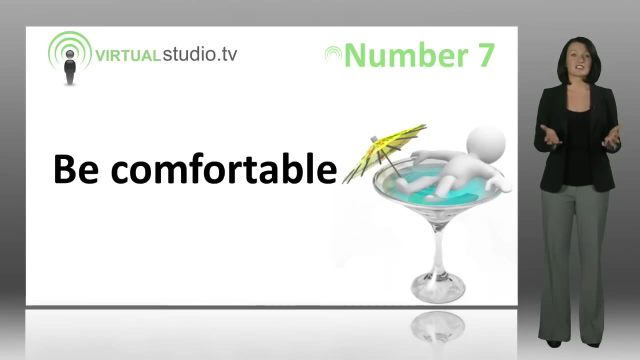 Number seven: make friends with yourself and be comfortable. Don't create a posher version of the real you, someone who uses big words and tries to disguise a regional accent. You are unique. You are special. Nobody is quite like you, So stick to the real you be authentic and the audience will. 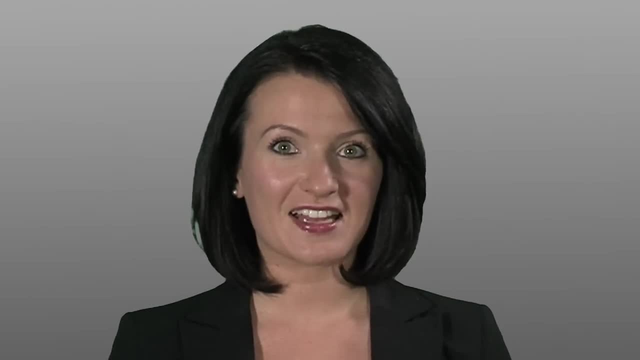 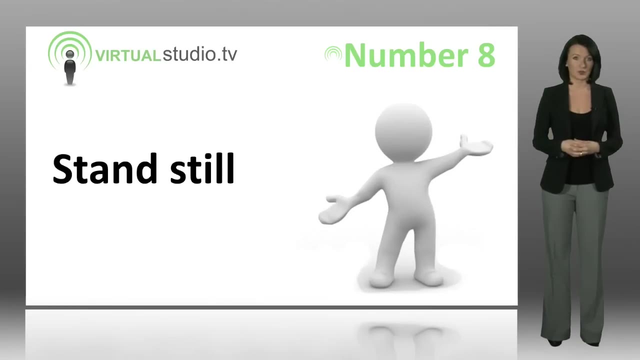 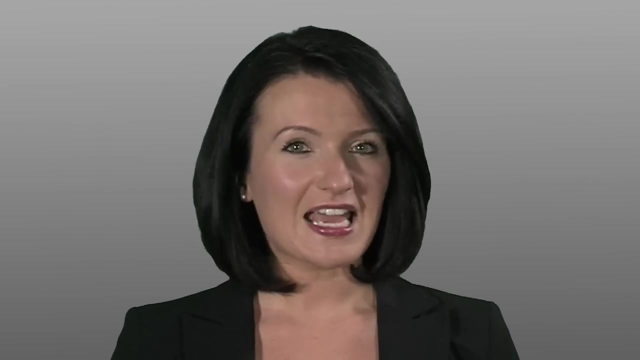 believe in you. Number eight stand still. Everyone feels a rush of adrenaline as they stand up ready to speak in front of an audience. As adrenaline flows through the body, your body will get ready for fight or flight. The lactic acid builds up in your muscle tissue and you will. 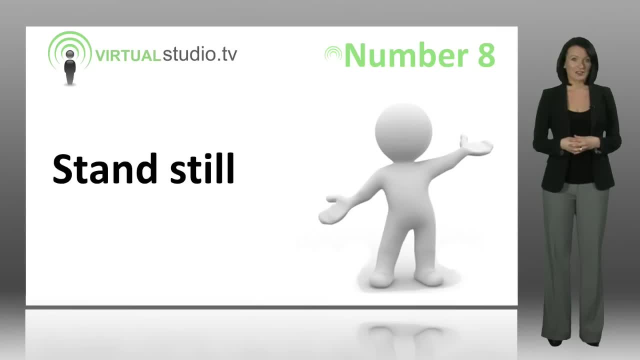 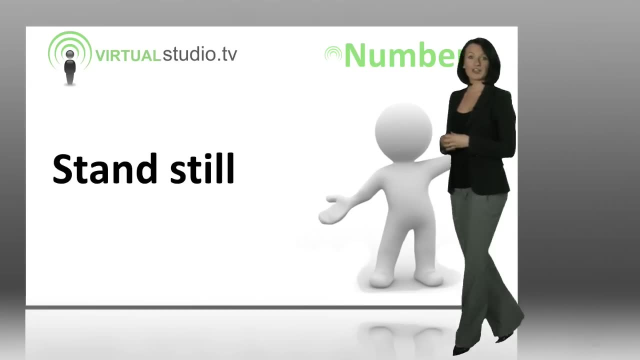 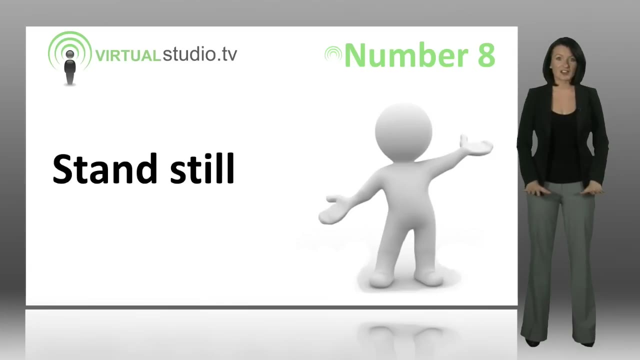 feel an overwhelming need to move. This is what we call weaving. An advanced stage of weaving is prowling from one end of the stage to the other. Lock out your hips and imagine that your feet are stuck to the floor. You still have plenty of room to move around. 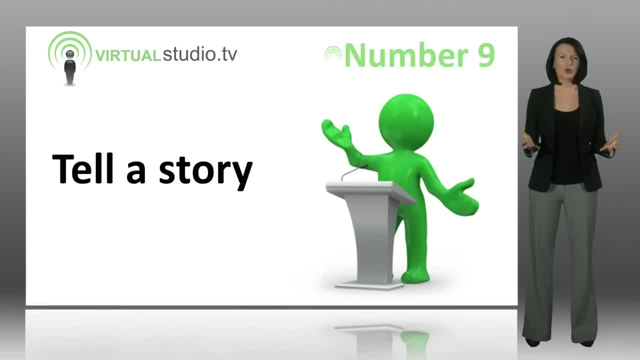 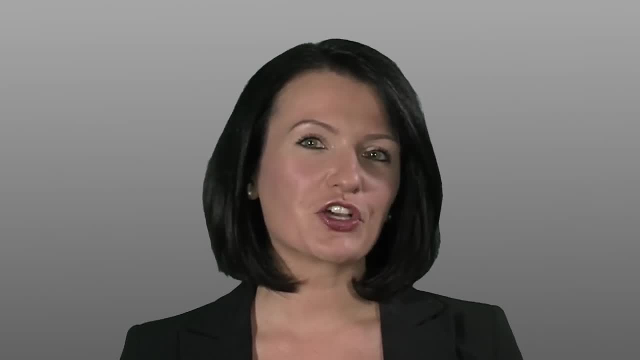 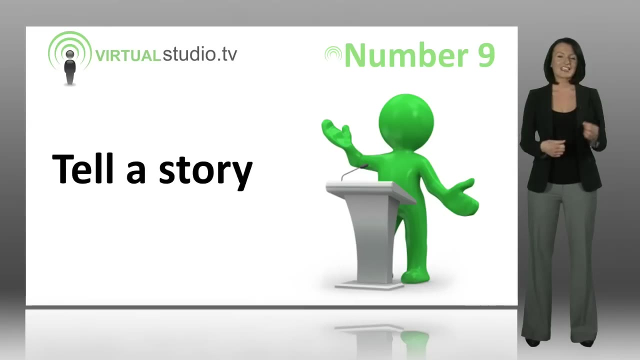 Number nine: tell a story. Forget the corporate spiel and all those text slides that no body will read. Tell the audience a story, Engage in a conversation with the audience and then, and only then, talk about targets and measurable goals. I guarantee you that the audience will remember a story that relates to your key messages.